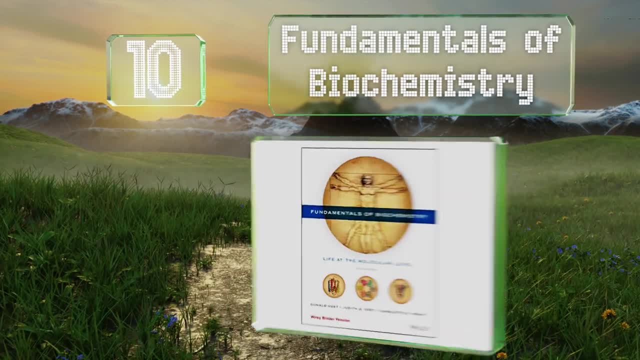 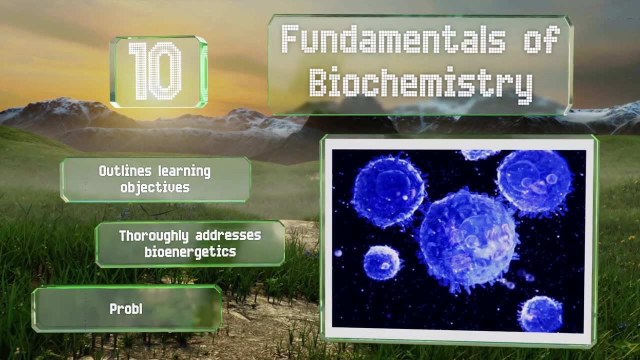 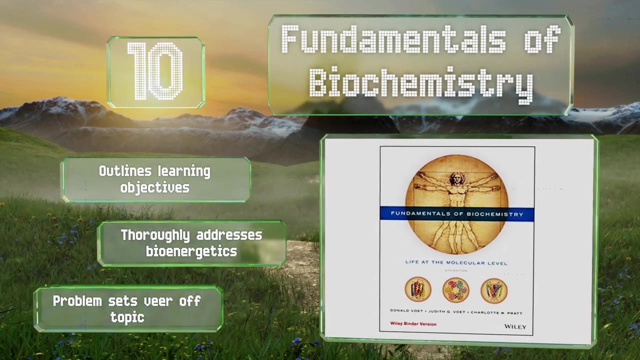 relating biochemical processes to their roots in chemistry. by way of even pacing, balanced coverage and straightforward explanations. It urges readers to think realistically about future challenges in the science. It outlines learning objectives and thoroughly addresses bioenergetics. However, the problem sets veer off-topic At number 9.. Charming and informative. 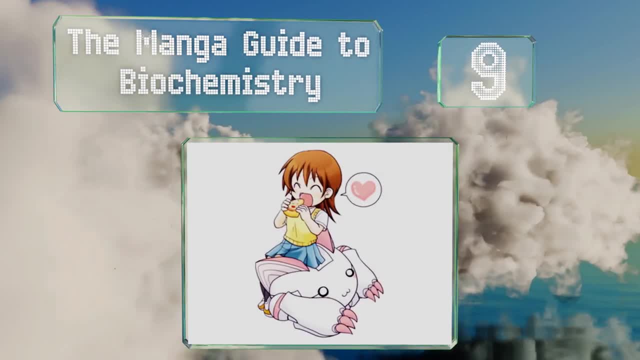 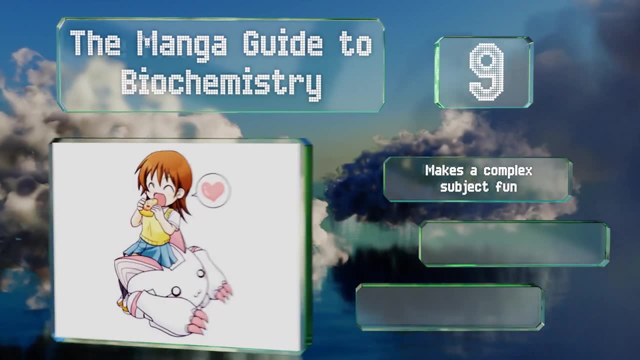 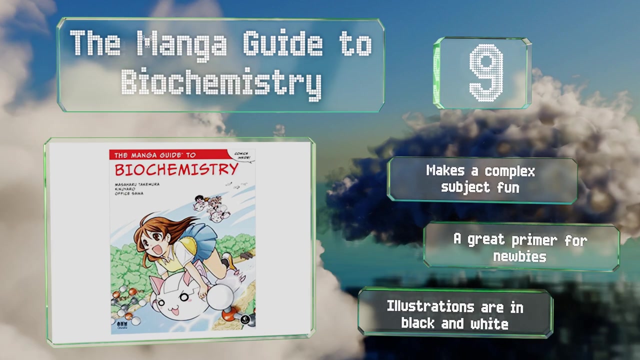 the Manga Guide to Biochemistry uses a character-driven storyline and a clever graphic novel format to educate readers on eventful biological processes such as the metabolism of carbohydrates and proteins, Enzyme kinetics and DNA transcription. It makes a complex subject fun and is a great 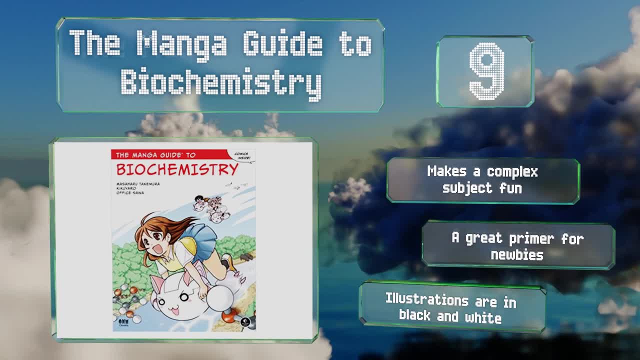 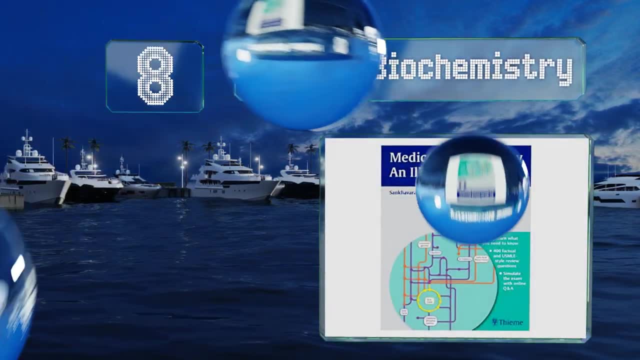 primer for newbies, But the illustrations are in black and white, Coming in at number 8 on our list, A good choice for visual learners. medical biochemistry boasts hundreds of full-color images of pathways, plenty of summary tables and handy color-coded 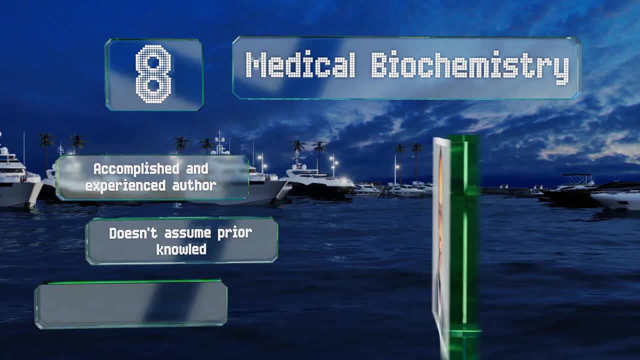 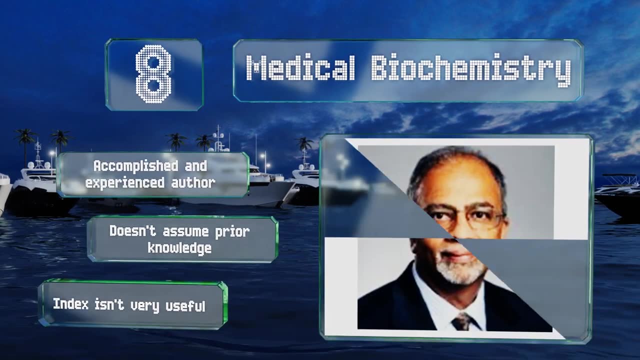 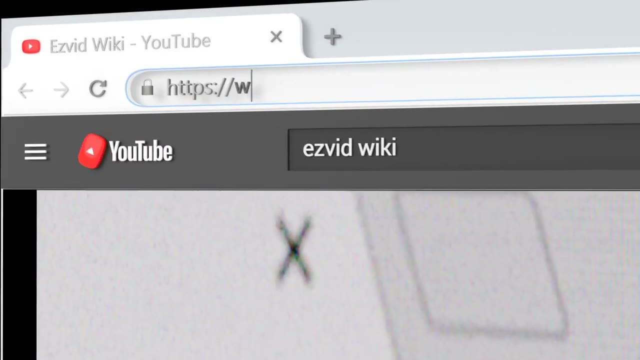 boxes. It strives to make meaningful connections between biochemical concepts and their related clinical conditions. It comes from a number of different sources, including the Manga Guide to Biochemistry, an accomplished and experienced author, and doesn't assume any prior knowledge. However, the index isn't very useful. Our newest choices can only be seen at wikieasybidcom. Go there. 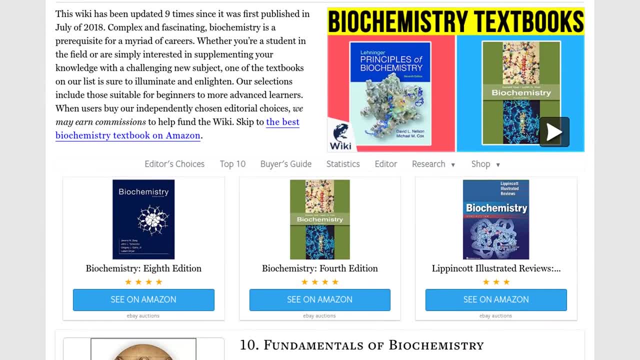 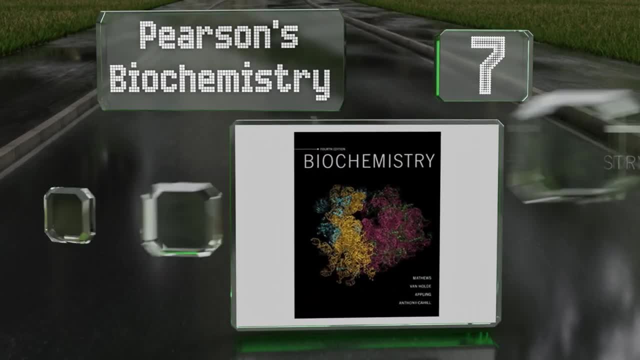 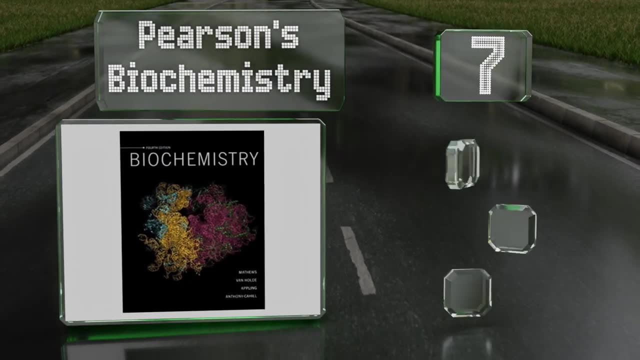 now and search for biochemistry textbooks, or simply click beneath this video At number 7.. In Pearson's Biochemistry, the authors seek to emphasize the experimental nature of the field and introduce nucleic acid structure early on in order to to illustrate protein functions. It uses a blend of contemporary insight and expertise to give 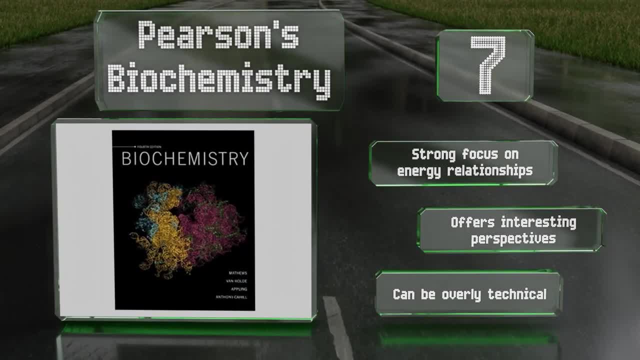 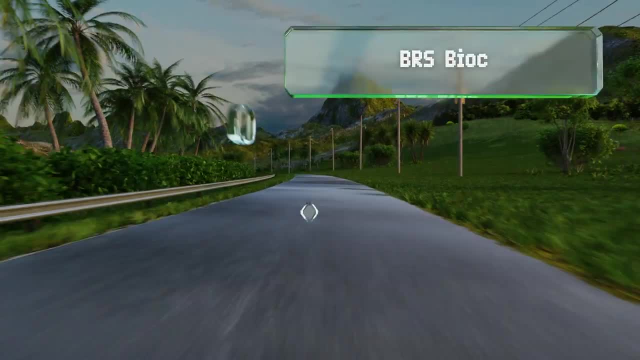 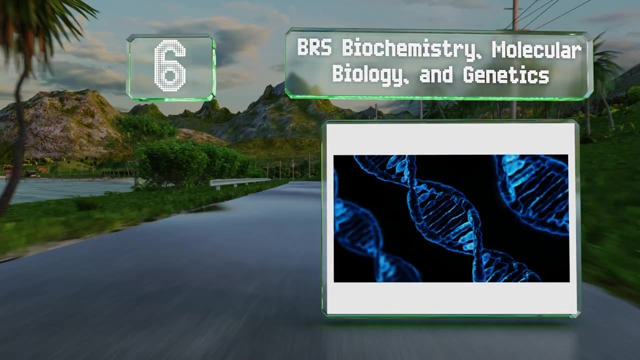 learners a solid grounding. It places a strong focus on energy relationships and offers interesting perspectives, but it can be overly technical. Moving up our list to number 6. BRS Biochemistry, Molecular Biology and Genetics serves as a constructive reference for those who need. 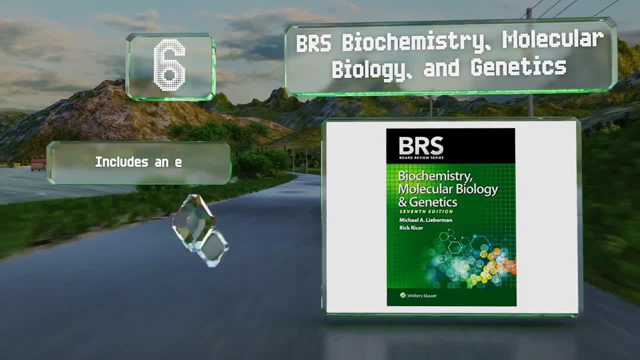 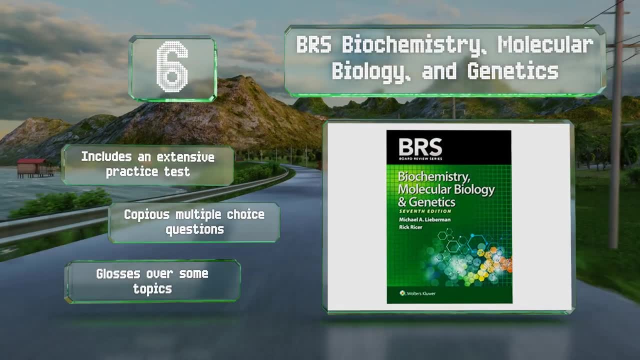 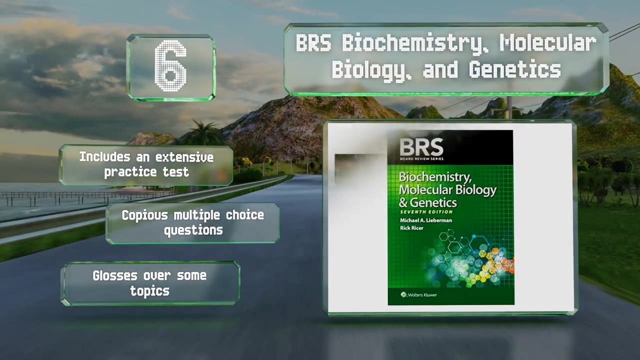 clarification. It covers myriad crucial topics using a succinct and accessible format, bolstered with pedagogical features that make it easy to follow. It includes an extensive practice test and copious multiple-choice questions. However, it glosses over some subjects Halfway up our list, at number 5.. Penned by husband and wife team Judith and Donald Vogt. 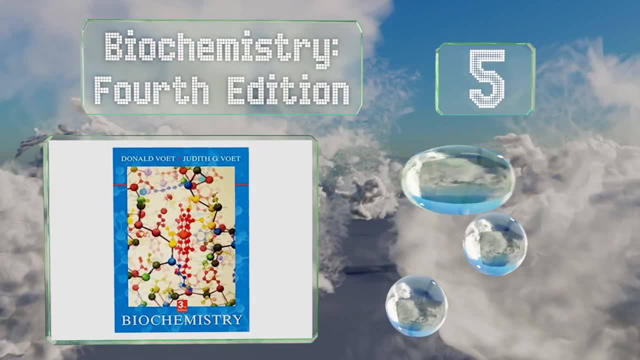 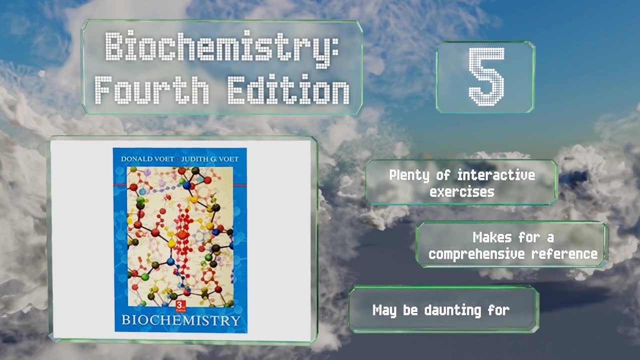 Biochemistry 4th Edition clears a high bar with both students and professors. Rich in detail, it uses a combination of classical and modern research to walk learners through evolutions- many variations. It contains plenty of interactive exercises and makes for a comprehensive reference. 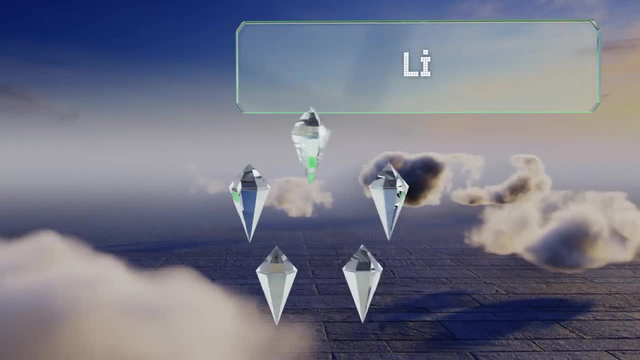 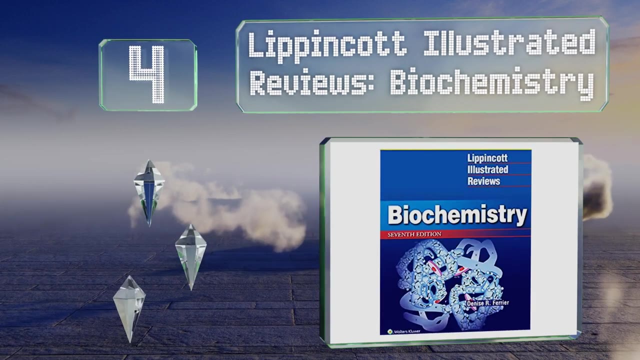 but it may be daunting for beginners At number 4. An invaluable study guide. Lippincott Illustrated Reviews Biochemistry uses a reader-friendly outline format to help students grasp material quickly to pass their exams Using no-fuss language. it covers key. 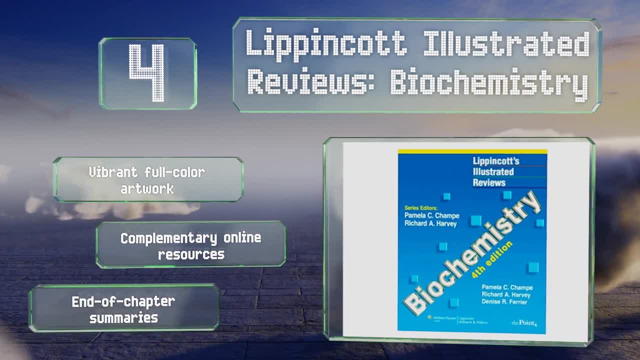 concepts with enough detail to reinforce without overwhelming. It features vibrant full-color artwork, complementary online resources and a wide range of materials. It's a great way to include a wide range of information, including a variety of materials, and it's a great way. 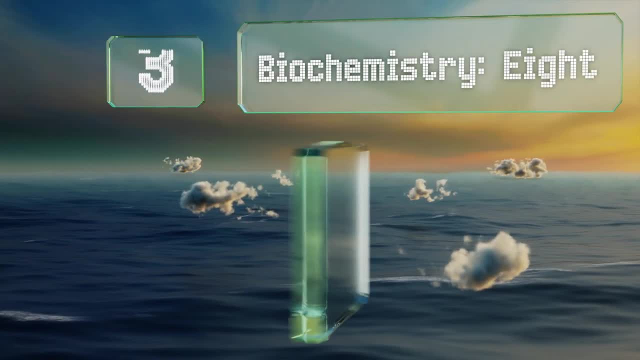 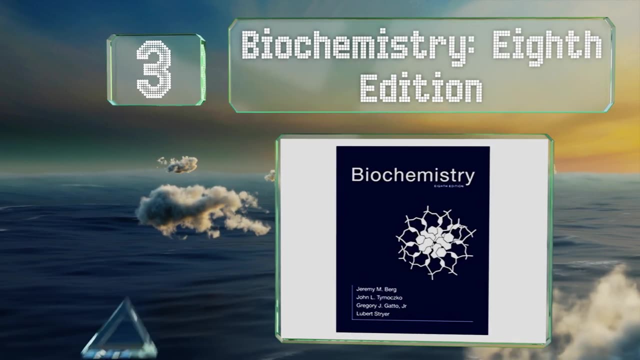 to include a variety of resources. It's a great way to include a variety of materials. End of chapter summaries, Niering the top of our list at number 3.. Biochemistry 8th Edition works to convey the complicated language of the field in a manner that's clear and concise, Chock, full of illuminating graphics. 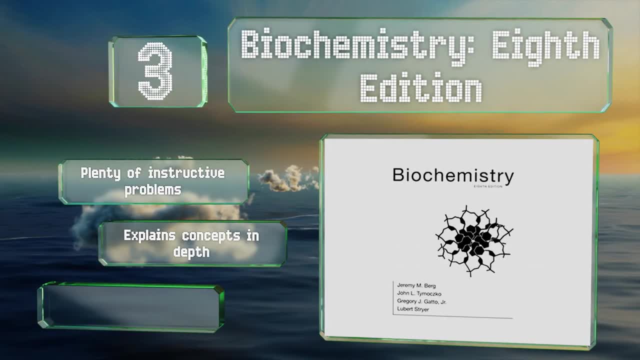 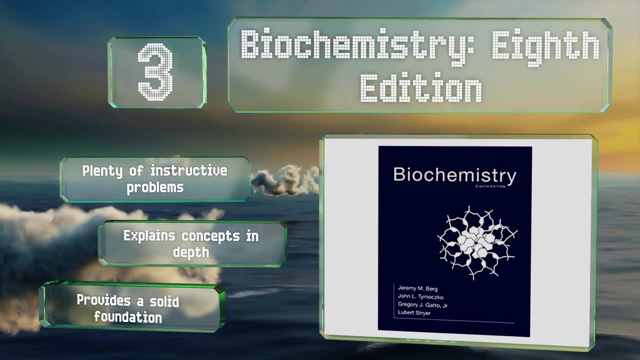 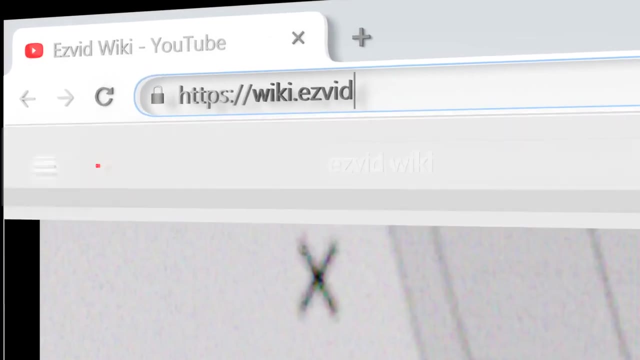 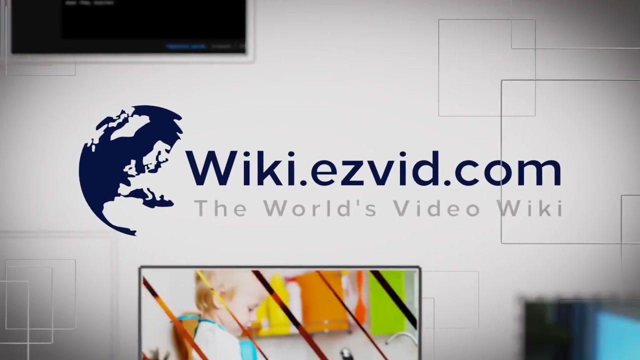 this authoritative text covers everything from advances in genetic regulation to helpful techniques for research. It includes plenty of instructive problems and explains concepts in depth. It provides a solid foundation. Our newest choices can only be seen by the audience at wikieasyvidcom. Go there now and search for biochemistry textbooks, or simply click beneath. 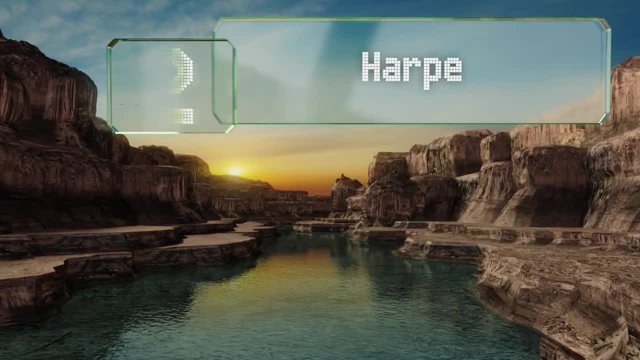 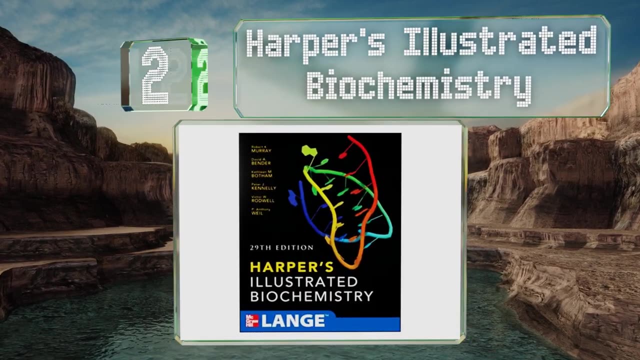 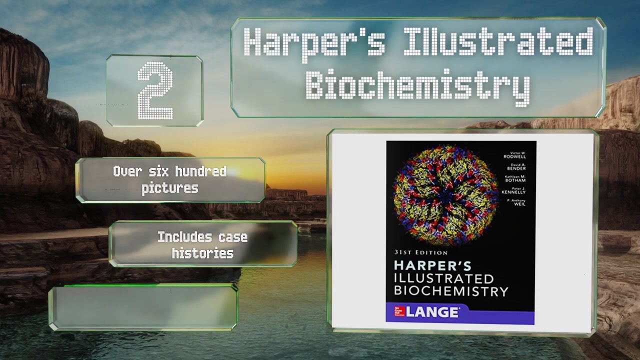 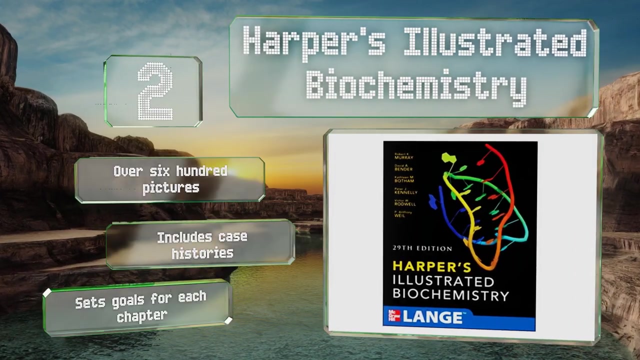 this video At number two, a great resource for aspiring healthcare professionals. Harper's Illustrated Biochemistry provides students with a full understanding of the discipline and its relation to clinical medicine, with an emphasis on disease diagnostic pathology and medical practice. It features over 600 pictures and case histories and sets goals for each chapter. 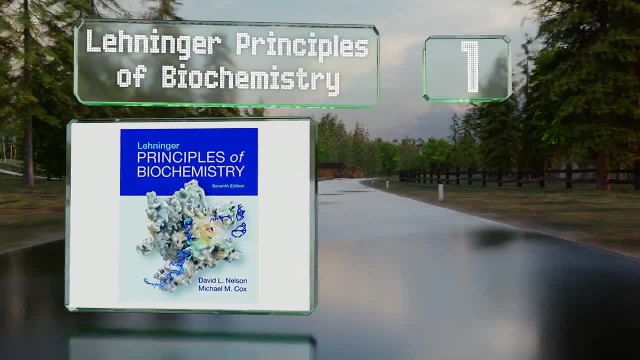 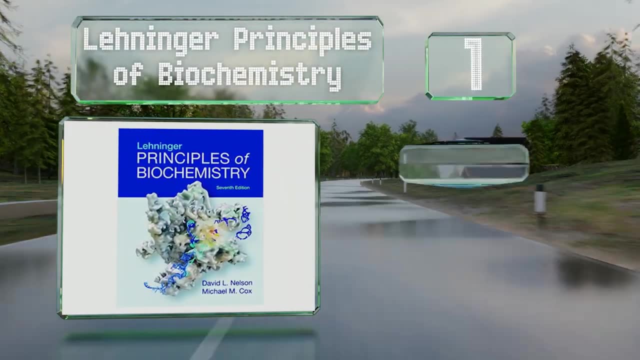 And taking the top spot on our list. in addition to its well-informed text, readers will appreciate the visually appealing layout of Leninger Principles of Biochemistry. It offers strategically placed graphics, bolded text and sidebars with relevant case studies that bring ideas to life. 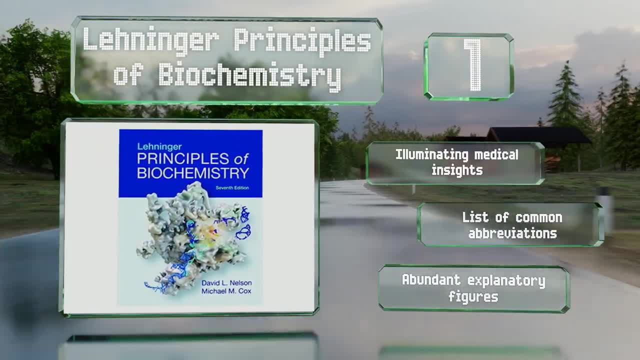 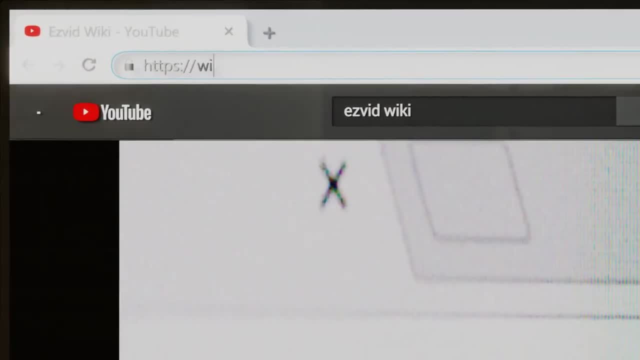 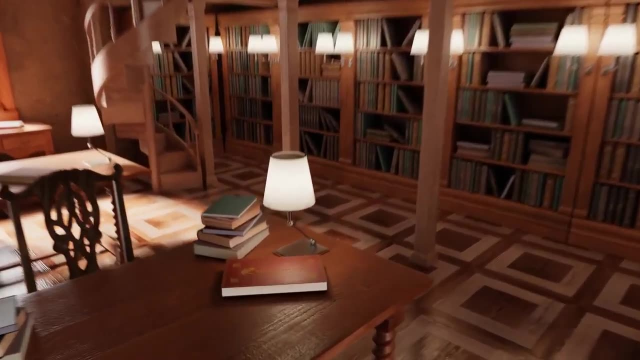 It includes illuminating medical insights, a list of common abbreviations and abundant explanatory figures. Our newest choices can only be seen at wikieasyvidcom. Go there now and search for biochemistry textbooks, or simply click beneath this video.